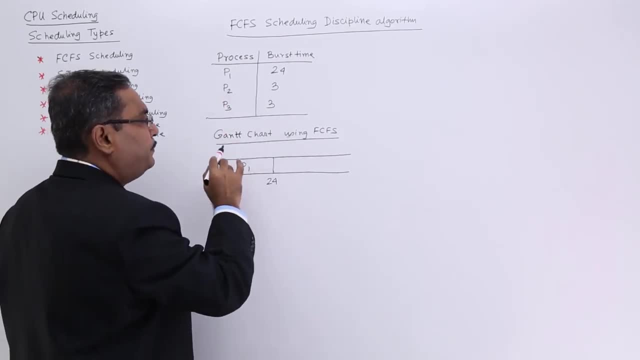 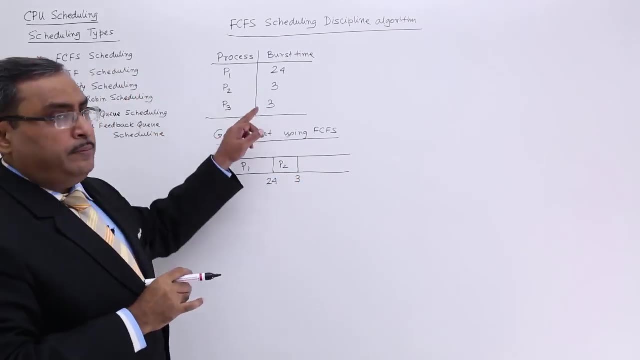 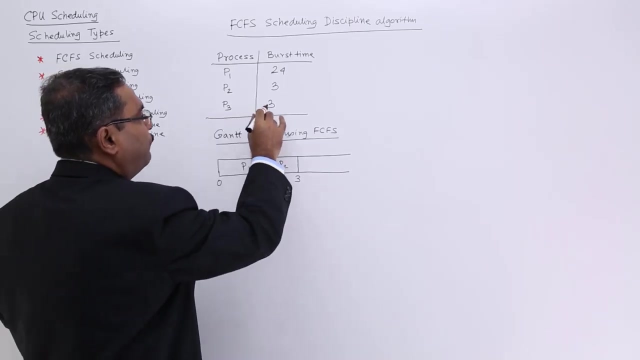 they are given in this order only. So now, then I shall go for P2, and P2 will have a burst time of 3 units. You know the burst time. Burst time means it is requiring- the time required to get complete. And then I shall for P3, and P3 will take another 3 units. 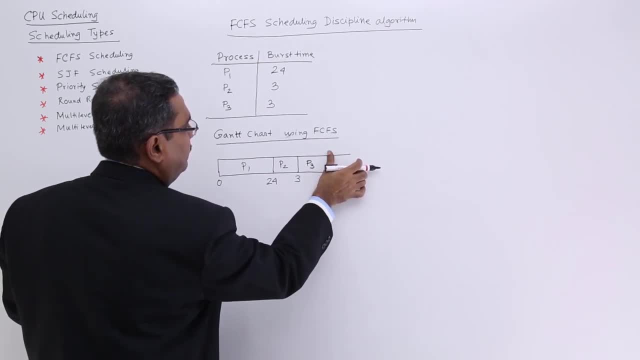 of time. So P3 is taking 5 minutes. So 5 minutes is the total time. 15 minutes is going. P3 will take another 3 units of time. so if I write this one as 27, here I am writing this: 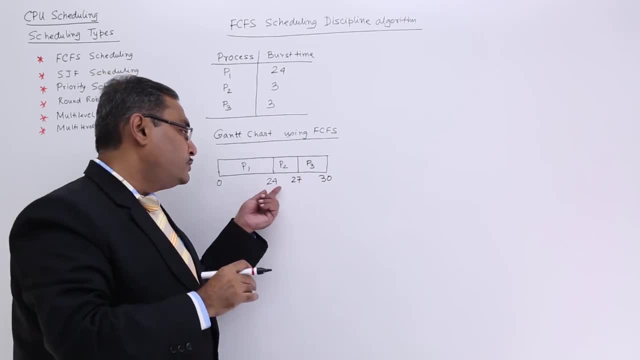 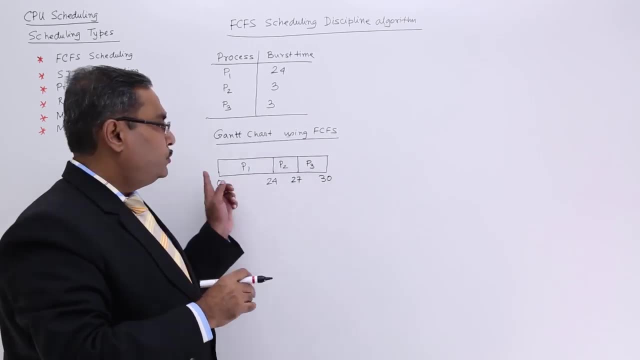 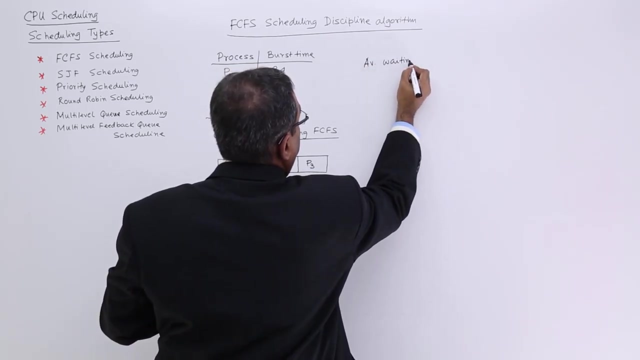 one as 30, because 3 units. I should not write 3 because I should go for this: 24 plus 3, 27, and then 27 plus 3, 30 will be the finishing time. so that is the total duration. so if we calculate the average now, we are going to calculate the average waiting time. how to? 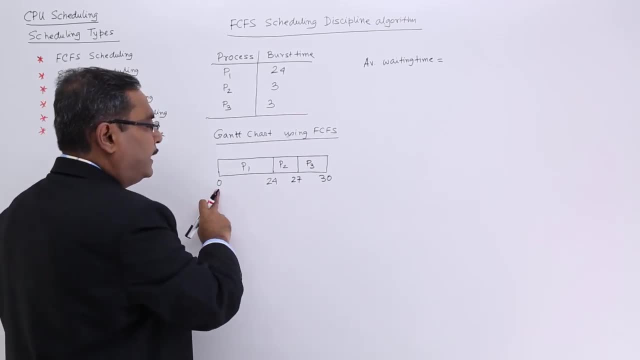 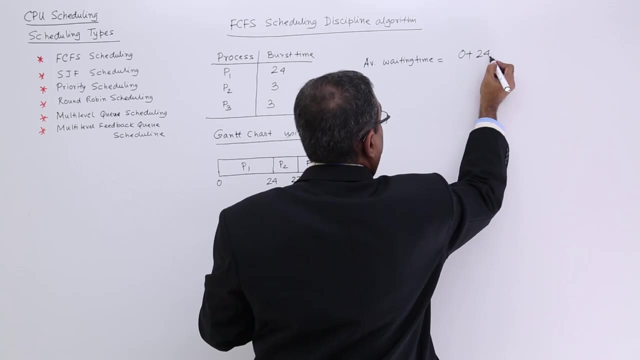 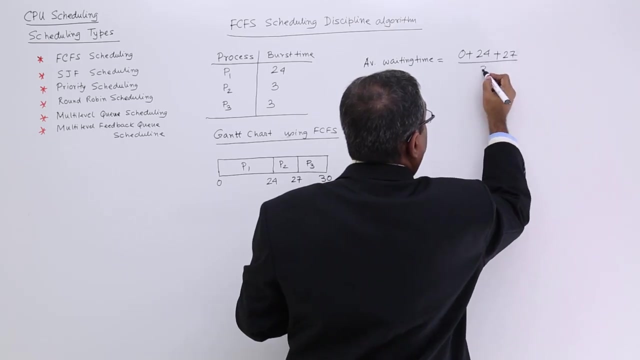 calculate the average waiting time. so now see for P1: there is no waiting time for P1. for P2, the waiting time is 24. now for P3, the waiting time is 27. so that is, the waiting time is 27. so now, if you go for the average waiting time for P2, the waiting time is 24. 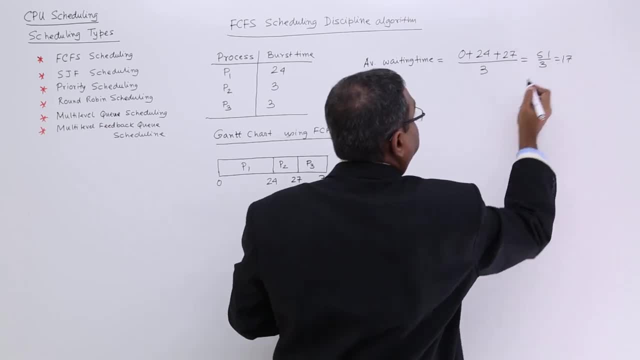 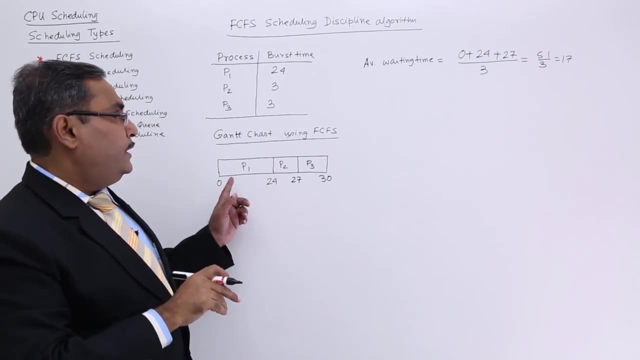 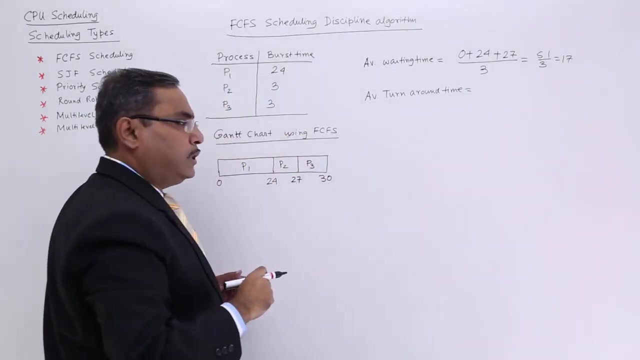 average. it is coming as this, So it is 17.. In this way the waiting time, average waiting time, can be calculated Here. you see, if you go for the turnaround time, say average turnaround time. So now it is the time between the submission and the completion. So for 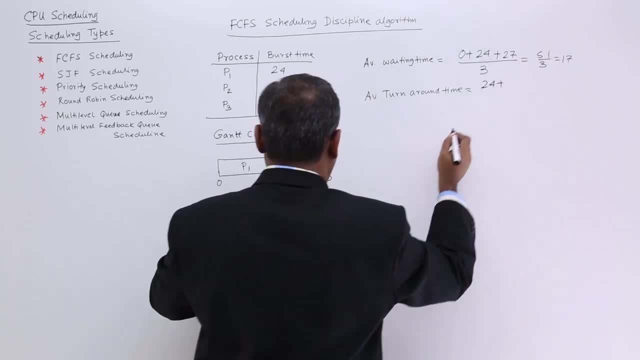 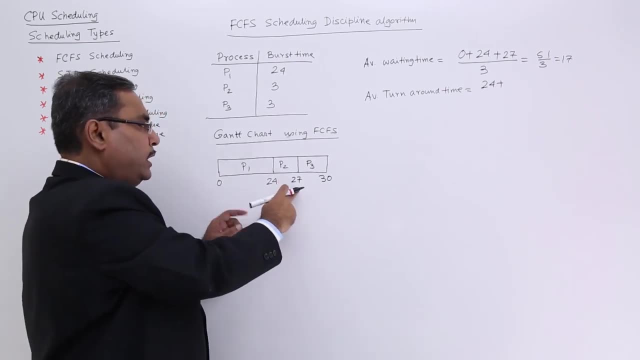 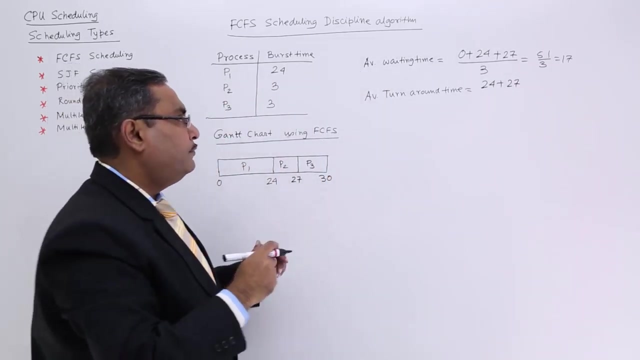 P1, the turnaround time is 24.. For P2, all of them have arrived, So that is why all of them were available from instance 0. So P2 will have the total turnaround time is 27. And P3 will have the turnaround time of 30. So if you do the calculation, then you 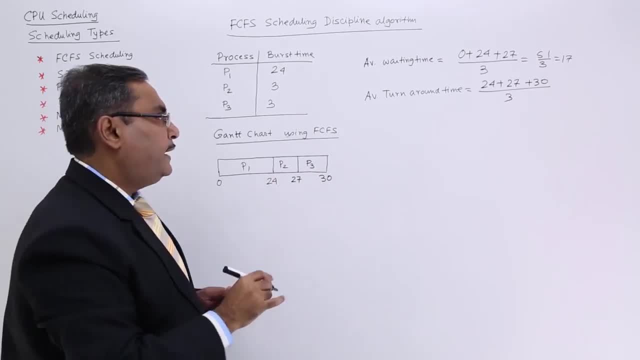 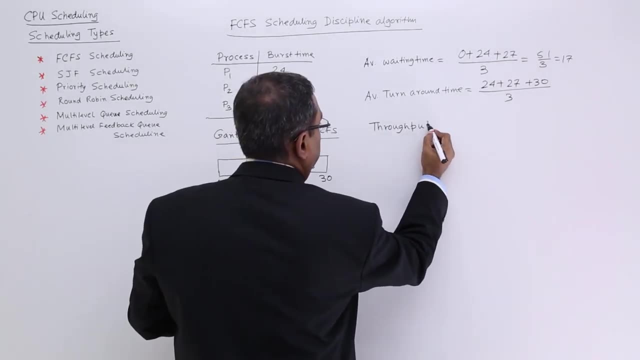 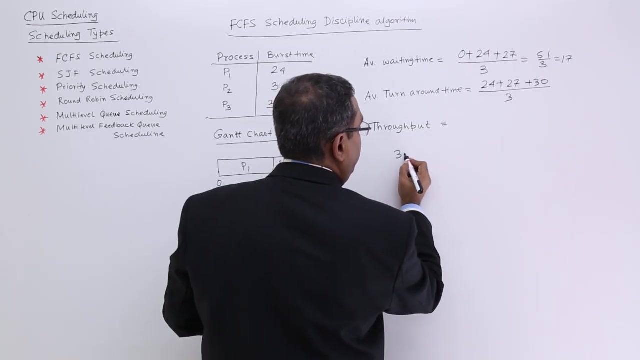 are getting the average turnaround time. Now if you calculate the throughput, throughput means number of Processes completed per unit time. So in 30 units I have completed 3 processes. So now if you go for 1 per unit time, So that is the throughput. So per unit means you. 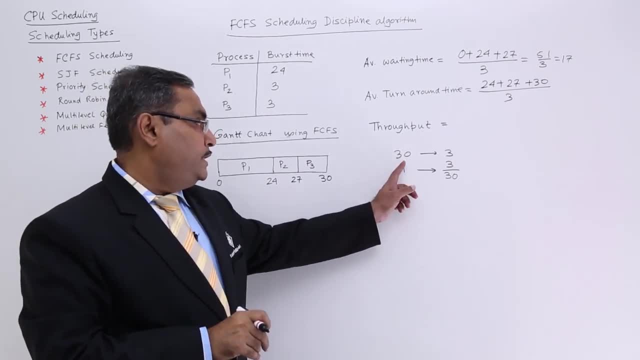 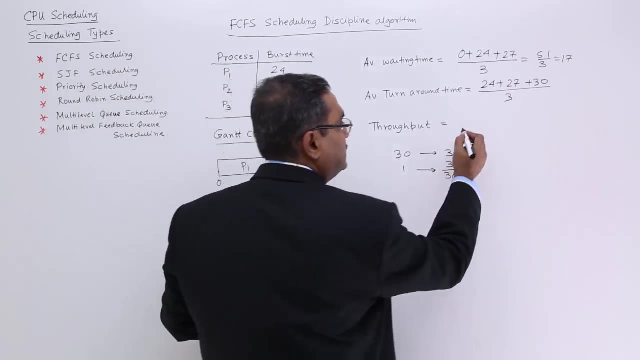 are going for unit time, So now out of 30, in this 30 units of duration. I have completed 3 processes, So 1 unit duration. I have completed these processes, So that means 3 bit of. 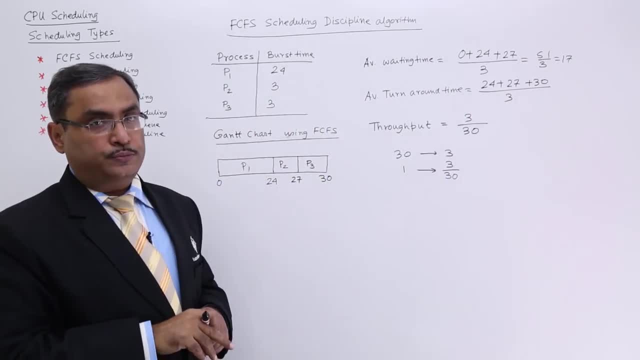 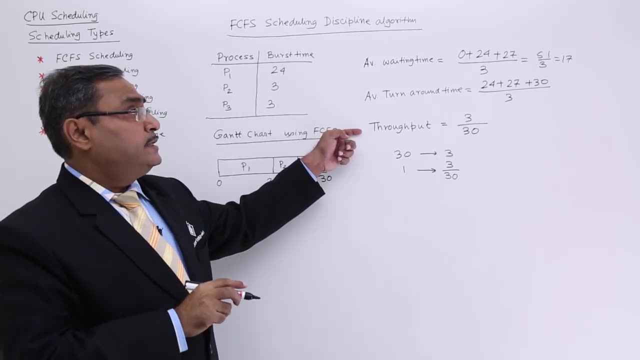 30 will be the duration. So that is my throughput. So now, in this way, the average waiting time, the turnaround time and this, they are working. In this case, the average waiting time and the response time will be the same, Because all the processes are having the response. 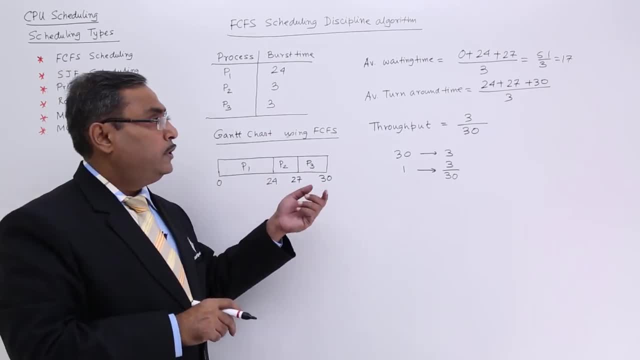 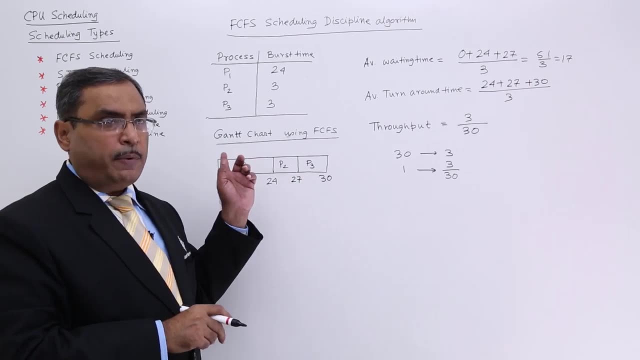 time is equal to the respective waiting time. So in this way I can do the calculations accordingly. So numerical problems will be coming in your gate exam on these particular scheduling disciplines. So you should have to do it, It is not necessary. 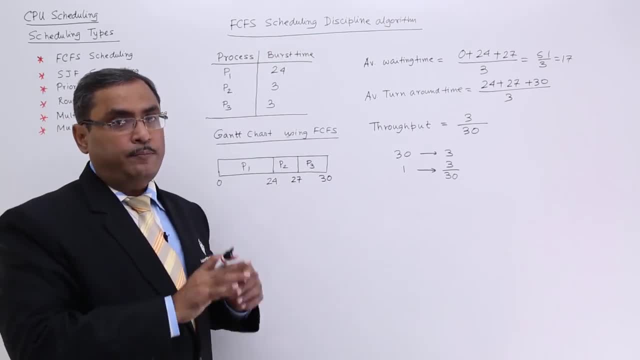 This is also very important. So you should have to do it. So you should have to do it, You should have to do it. So in this way, you should have to do it, You should have to do So. you should have to answer them properly. 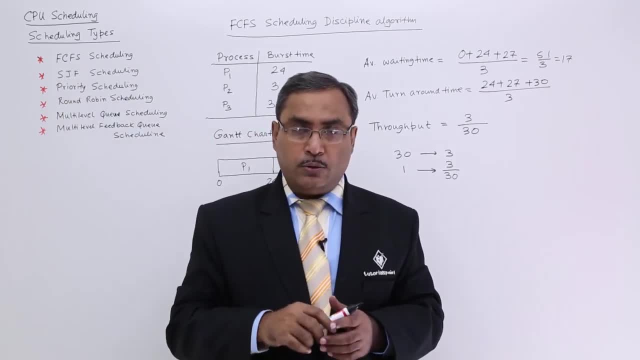 I think you have got the logic. how did I calculate this particular values? Thanks for watching this video. 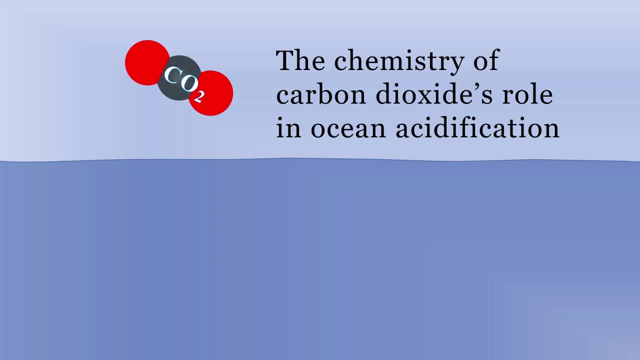 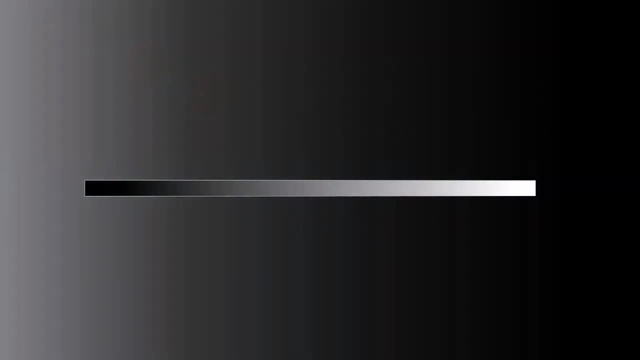 Hello and welcome to the chemistry of carbon dioxide's role in ocean acidification and its effects on ocean life. First let's take a look at what we mean by acid, And we can look at this bar as a continuum on the left showing low amounts of dissolved hydrogen ions, and on the